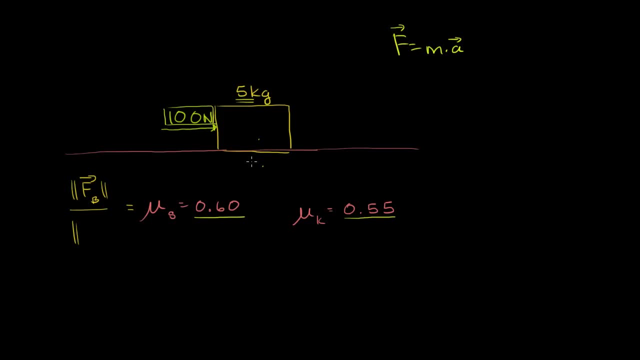 is the same thing as the normal force that the ground is applying on the block, The magnitude of the normal force that the ground is applying on the block. Then, once it's moving, then we could say that this is going to be, that this will. then. 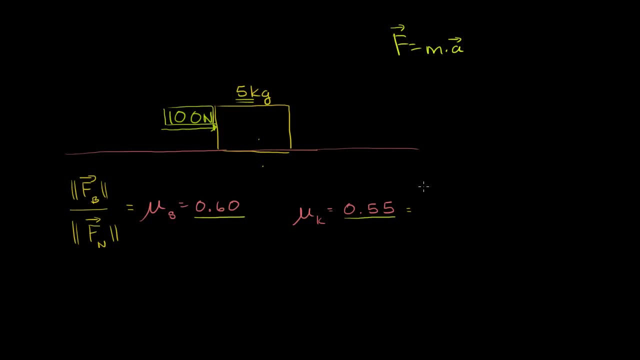 be equal to the force. This over here will be equal to the force of friction. So this is the force that's going to overcome friction, And then this over here will be equal to the force of friction. the magnitude of the force of friction. 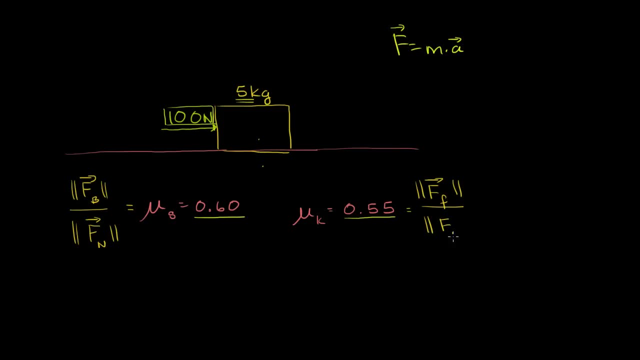 over the force of contact, the contact force between those two, So over the normal force. And it makes sense that the larger the contact force, the more that these are being pressed together, the little- at the atomic level they kind of really get into each other's grooves- the more 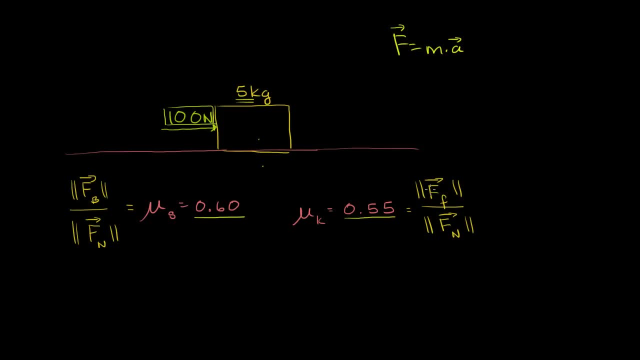 budging force you would need Or the more friction force would go against your motion. And in either situation the force of friction is going against your motion. So even if you push it on that way, it's not like force of friction is all of a sudden. 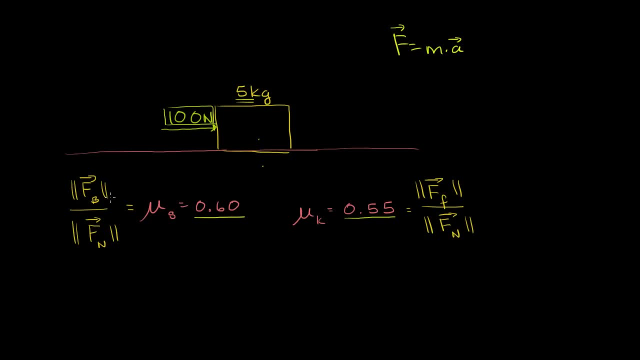 going to help you. So let's think about what the necessary force we need to do to overcome the force of friction right here in the static situation. So the force of gravity on this block is going to be the gravitational field, which is 9.8 meters per second. 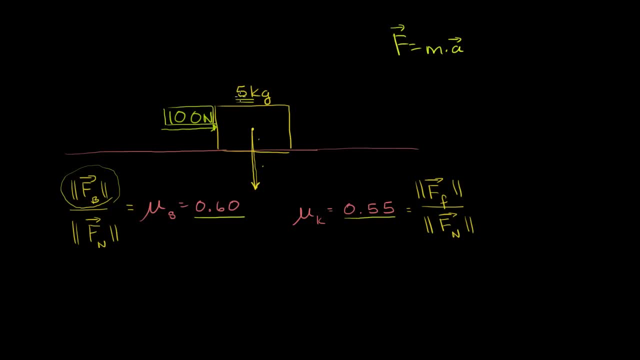 Times 5 kilograms: 9.8 meters per second. times 5 kilograms gives us 49 kilogram meters per second, or 49 newtons down. This is the force, the magnitude of the force. due to gravity, The direction is straight down towards the center. 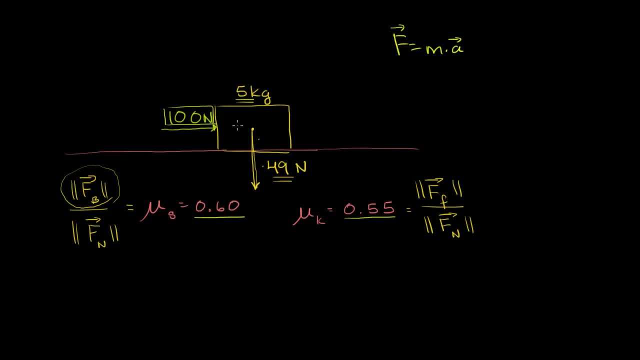 of the Earth, The normal force. and that force is there because this block is not accelerating downwards. So there must be some force that completely balances off the force of gravity And in this example it is the normal force, So it is acting 49 newtons upward. 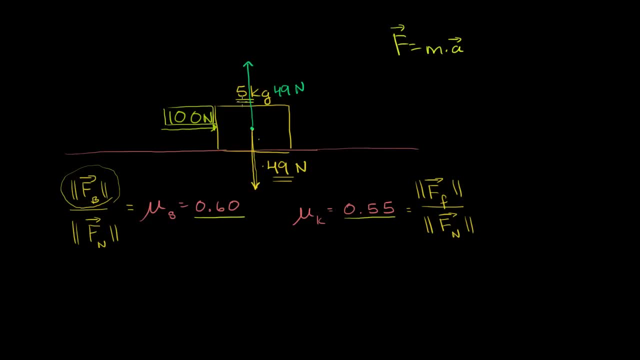 And so these net out, and that's why this block does not accelerate upwards or downwards. So what we have is the magnitude of the budging force needs to be equal to over the magnitude of the normal force. Well, this thing right over here is going to be 49 newtons. 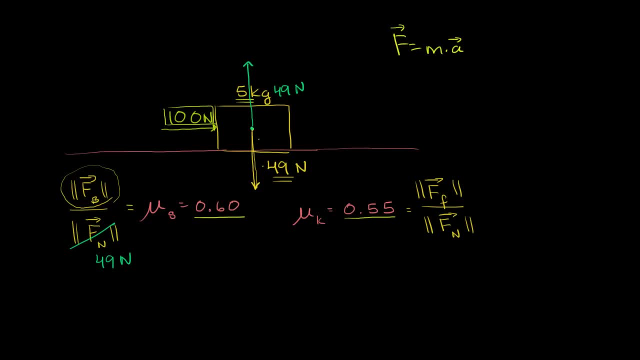 is equal to 0.60.. Or we could say that the magnitude of the budging force is going to be equal to 49 newtons times the coefficient of static friction, or that's 49 newtons times 0.60.. And remember, coefficients of friction are unitless. 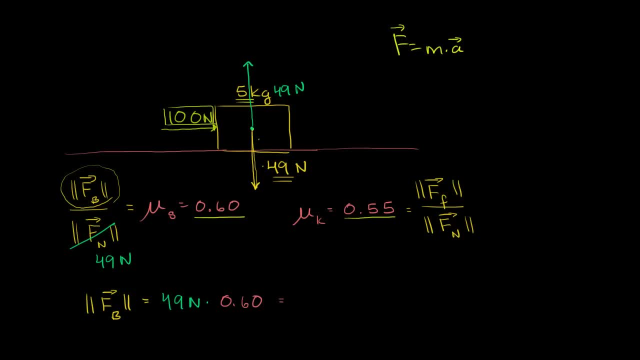 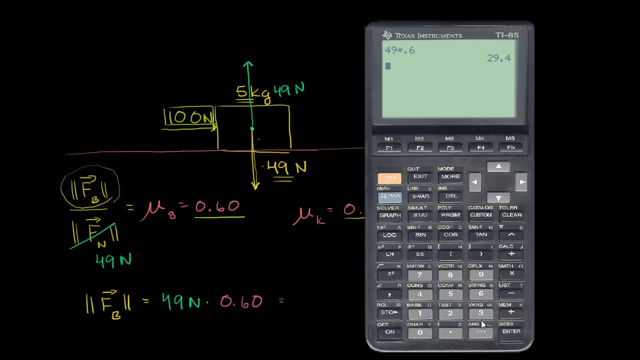 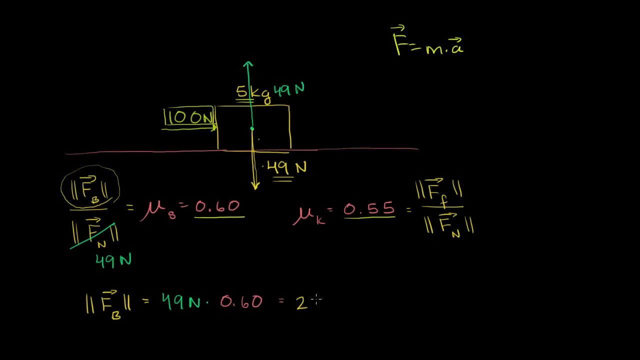 So the units here are still going to be in newtons, And so this gives us get out our calculator. this gives us 49 times 0.6, gives us 29.4 newtons. This is equal to- let me write it- 29.4 newtons. 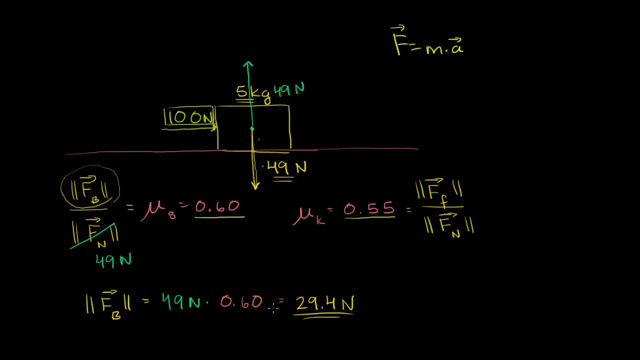 So that's the force necessary to overcome static friction, which we are applying more than enough of. So with 100 newtons, we will just start to budget And right when we're just at that moment where the thing is just starting to move, the net force. so we have 100 newtons. 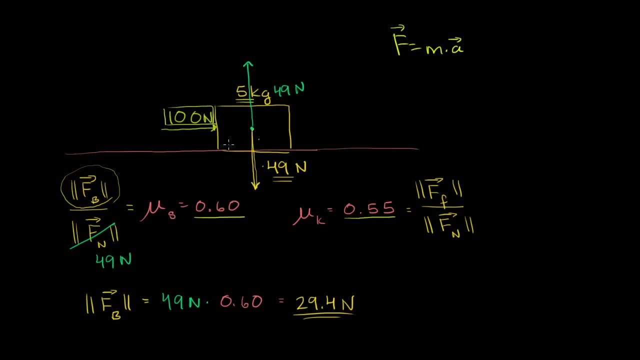 going in that direction and the force of static friction is going to go in this direction. Maybe I could draw it down here to show it's coming from the other direction. Maybe I could draw it from right over here. The force of static friction is going to be 29.4 newtons. 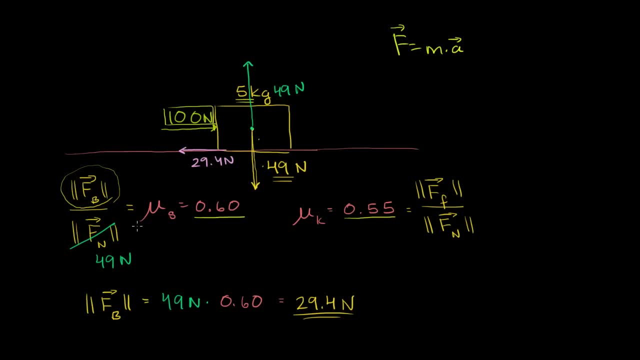 that way. And so right, when I'm just starting to budget this, just for that little moment, because once I do that, then all of a sudden it's moving and then static friction, or, sorry, kinetic friction, starts to matter. But just for that moment I'll have a net force of 100 minus. 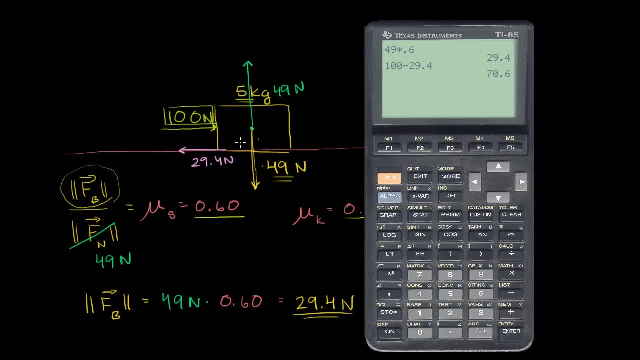 29.4 to the right. So I'll have a net force of 70.6.. So I will have a net force of 70.. What did I just write there? 70.6.. I could do that in my head. 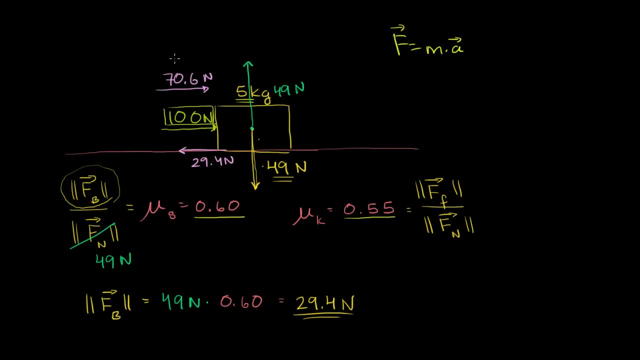 I shouldn't have to look at that 70.6 newtons for just a moment while I budget. So, just exactly, while I'm budgeting it, while we're overcoming the static friction, we have a 70.6 newton net force in the right direction. 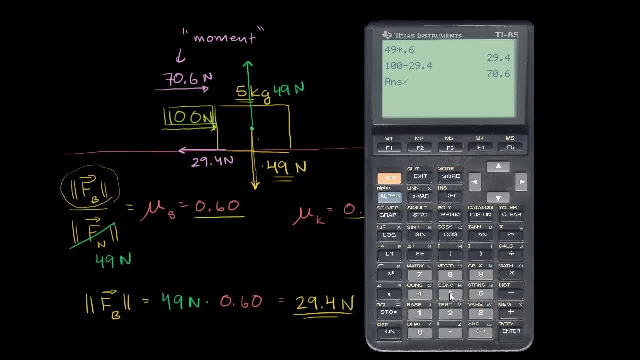 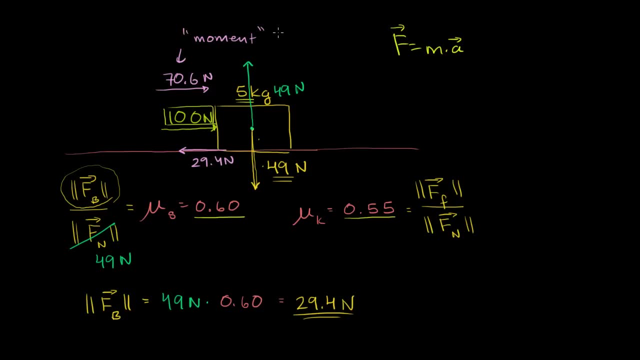 And so, just for that moment, you divide it by a 5 kilogram mass, So just for that moment it'll be accelerating at 14.12 meters per second. So you'll have an acceleration of 14.1 meters per second. 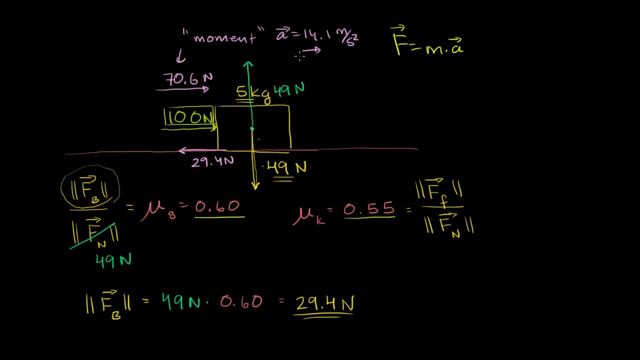 squared to the right. But that will just be for that absolute moment, because once I budget, all of a sudden the block will start to be moving, And once it's moving the coefficient of kinetic friction starts to matter. We got the things out of their little grooves. 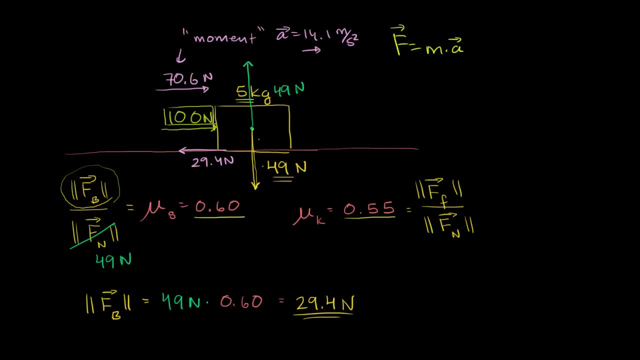 and so they're kind of gliding past each other on the top, although there still is resistance. So once we budget, we'll have that acceleration for just a moment. Now, all of a sudden, the coefficient of kinetic friction comes to play. 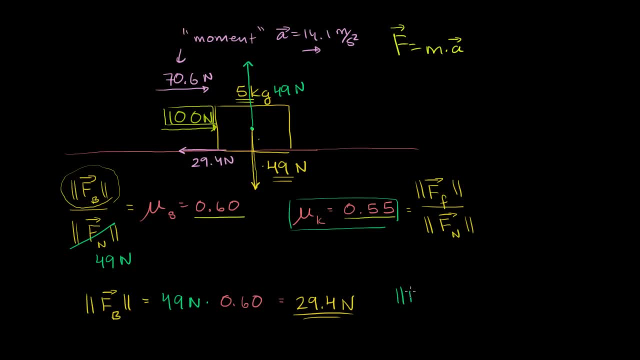 And the force of friction, assuming we're moving the force, the magnitude of the force of friction, it'll always go against our movement is going to be. remember: our normal force, we already said, is 49 newtons. 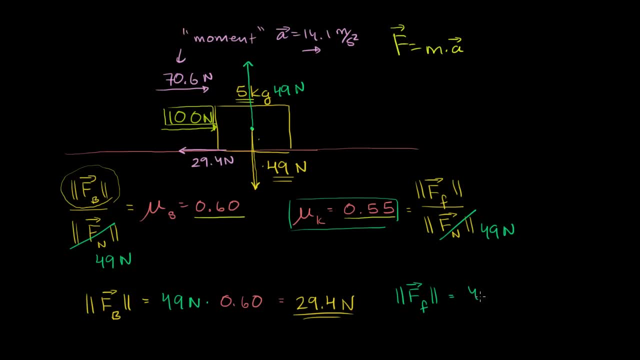 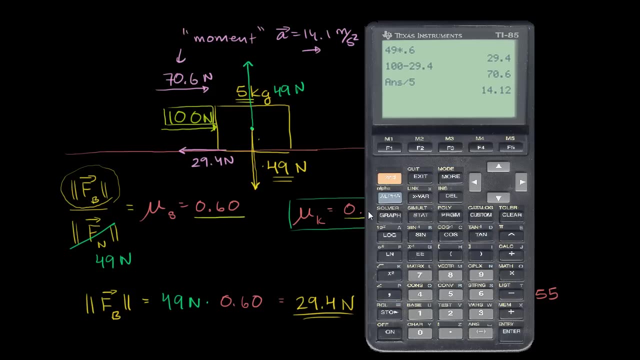 So it's 49.. We multiply both sides of this times 49. You get 49 newtons times 0.55, which is equal to 49 times 0.55, is equal to 26.5.. So this is equal to 26.95 newtons. 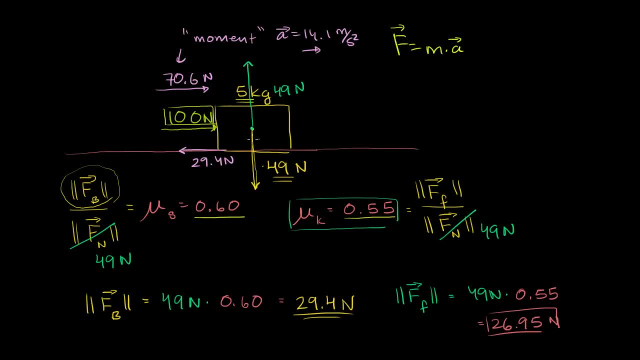 This is the force of friction, This is the magnitude, and it's going to go against our motion. So as soon as we start to move in that direction, the force of friction is going to be going in that direction. So once we start moving- assuming- 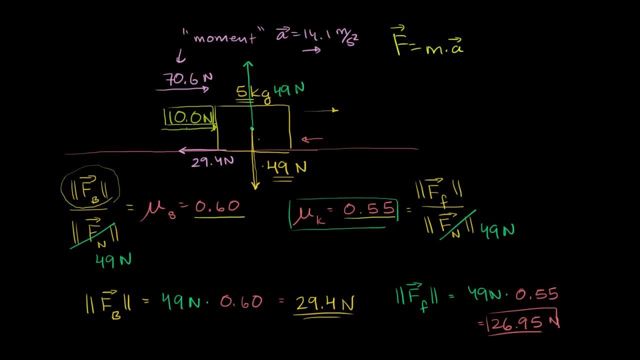 that I'm continuing to apply this 100 newtons of force. what is the net force? So I have 100 newtons going that way and I have 26.95 newtons going that way. And remember, with vectors I don't have to draw them here. 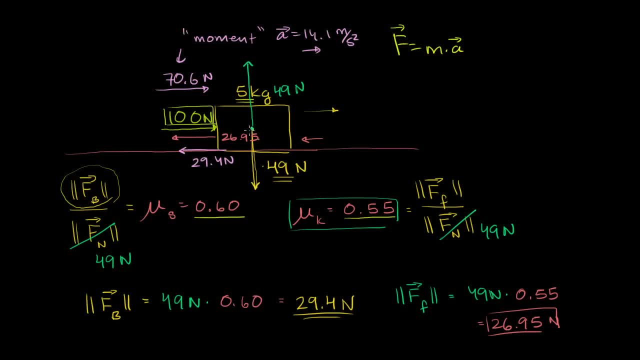 I could draw all of them, so all of their tails start at the center of mass of this object. I could draw them whenever, But remember, this is acting on the object, So it's usually, if you want to be precise, you'd show it- acting on the center of mass. 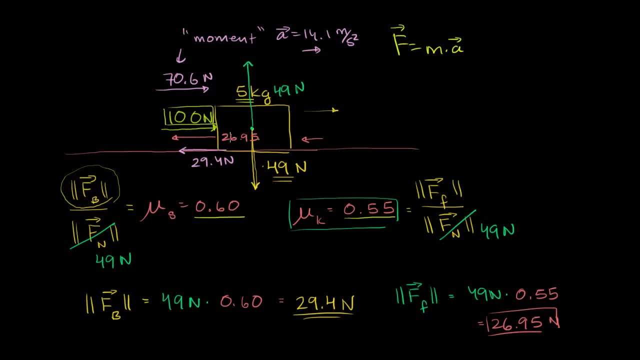 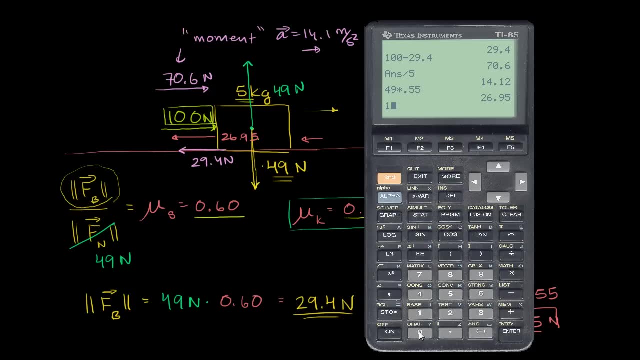 because we can view all of these atoms as one collective object. But anyway, what is the net force now? Well, you have 100 newtons to the right. You have 26.95 newtons to the left, 100 minus 26.95.. 100 newtons to the right. 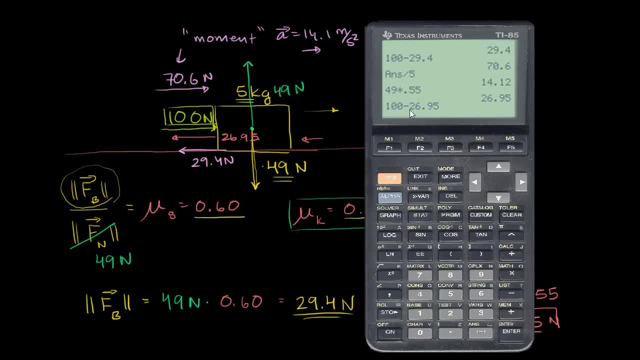 So you have 26.95 newtons to the left. So you have 26.95 newtons to the left, 100 minus 26.95.. 100 newtons to the right, 100 newtons that I'm applying to the right. 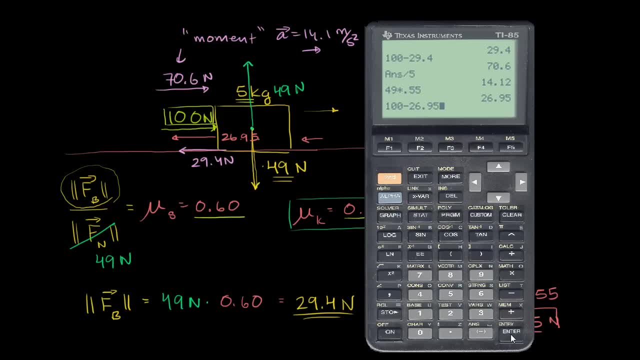 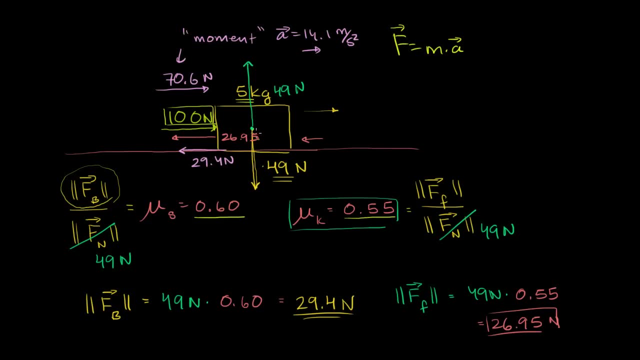 Minus 26.95 newtons, which is the force of friction to the left, always acting against us, means that there's a net force to the right of 73.05.. So once we're moving, we have a net force.